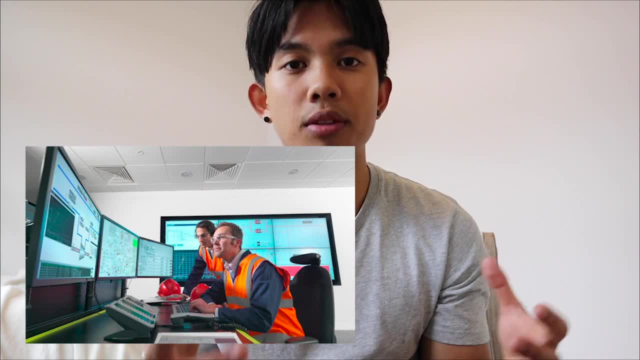 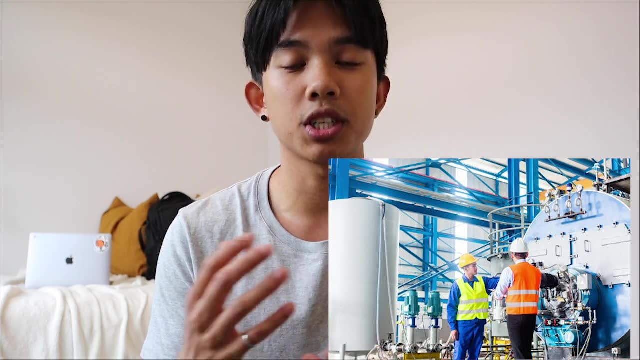 system data to figure out what is going on, maybe around the different equipment surrounding that thing. If you can't figure it out quickly, maybe you'll have to design a set of experiments to figure out what went wrong. If things are going well, maybe you can look into different optimization. 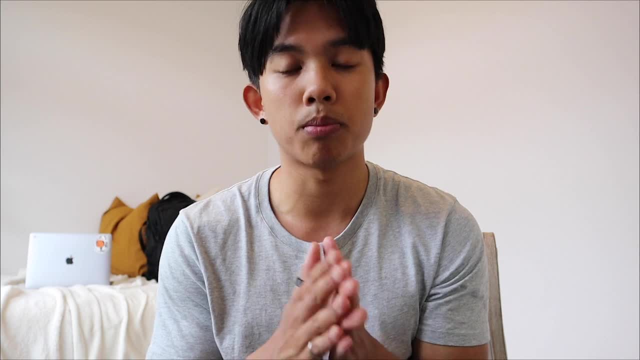 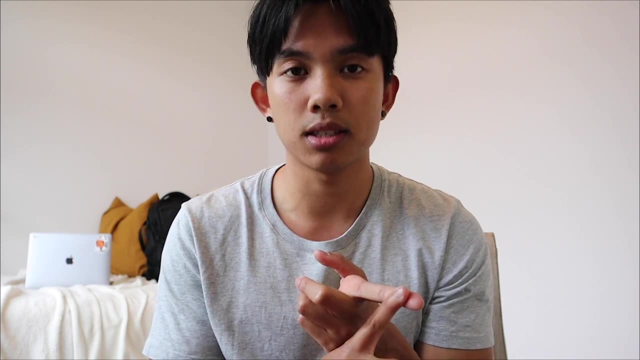 projects. Chemical engineers are constantly thinking about how we can improve the processes that we manage. Before you make any changes in the plant, you really have to come up with a detailed set of economic analyses- feasibility analysis- to make sure that you don't ruin anything else in the 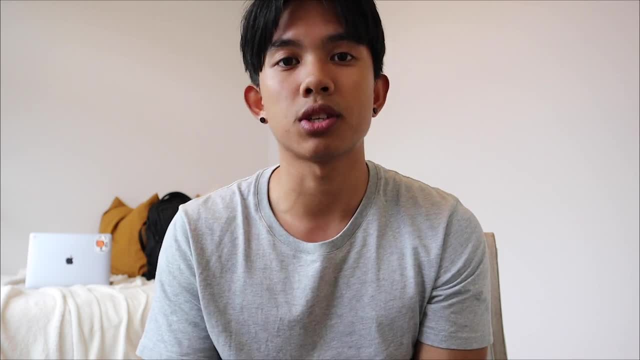 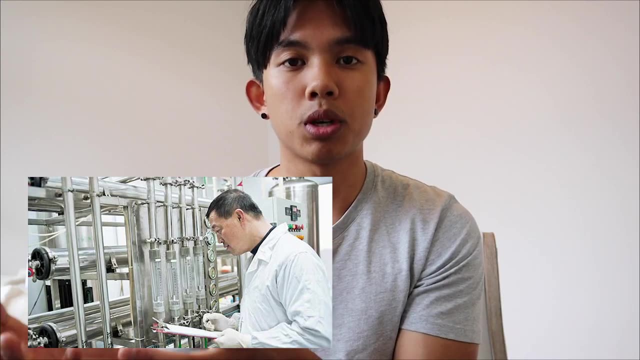 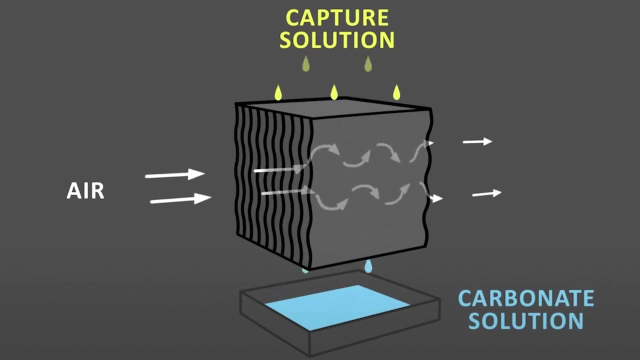 plant, And some of these capital projects can take years to install. In more research and development-based roles, you could be looking into how to scale up chemical process from the lab scale all the way up to commercial scale. New processes like direct air capture, hydrogen fuel cells and other alternative energies are constantly being 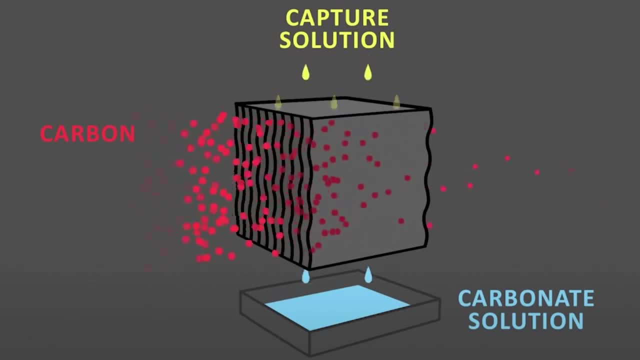 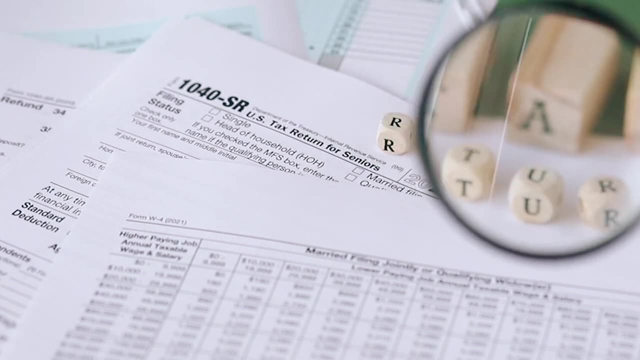 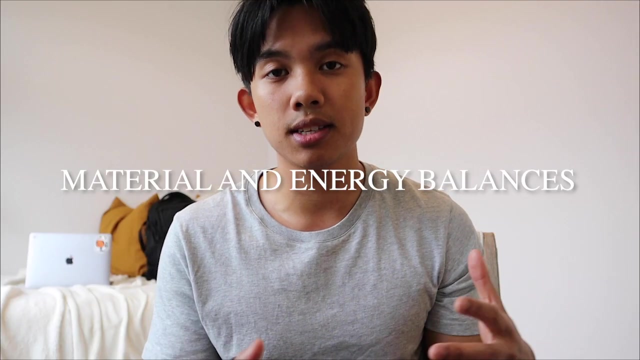 researched and developed into larger scale processes. Your first course object in chemical engineering will be material and energy balances. Just like a company has financial statements to keep track of the money flowing in and flowing out of the company, to determine their overall profitability, a chemical engineer has to take into account the ins and outs of a plant to make sure that the overall 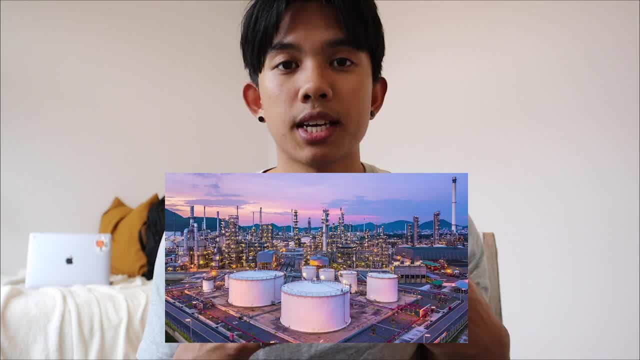 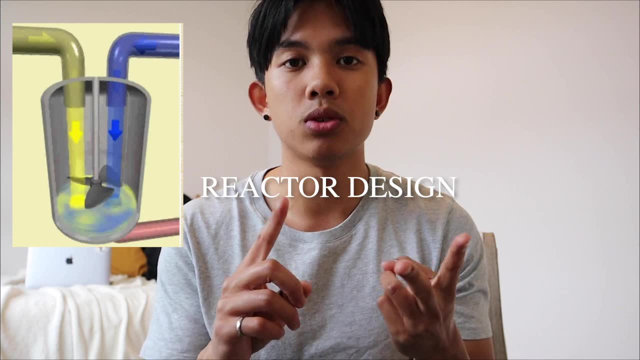 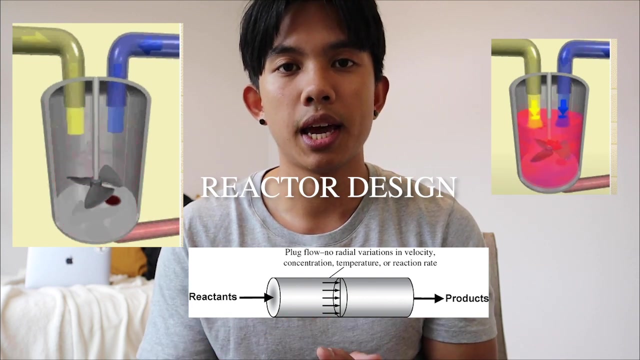 system is efficient. At the core of every chemical process is a reactor. In reactor design, you'll learn about the different equations governing these chemical reactors, from batch reactors to continuously stirred reactors to plug flow reactors. Each of these reactors can be applied to a different chemical process and you'll learn about how to optimize these different types of 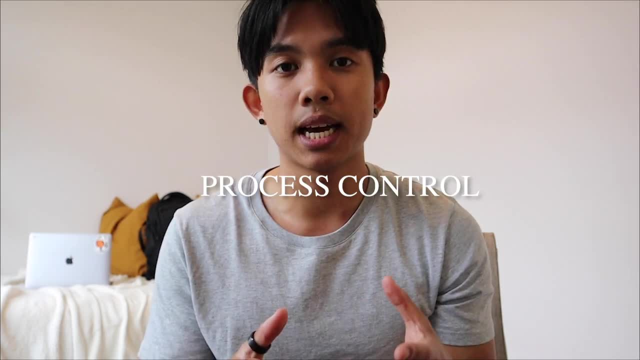 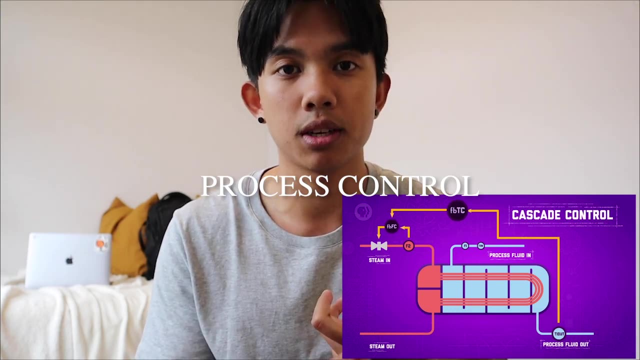 reactors Next up. we have process control. Every piece of equipment at the plant has a certain temperature, pressure and temperature. Each of these reactors has a different temperature, pressure and temperature. Each of these reactors has a certain temperature, pressure and temperature. This requires. 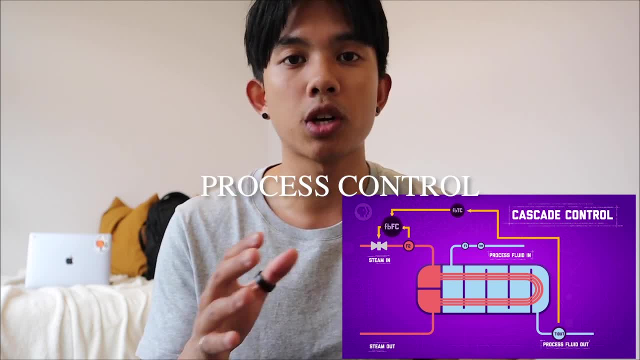 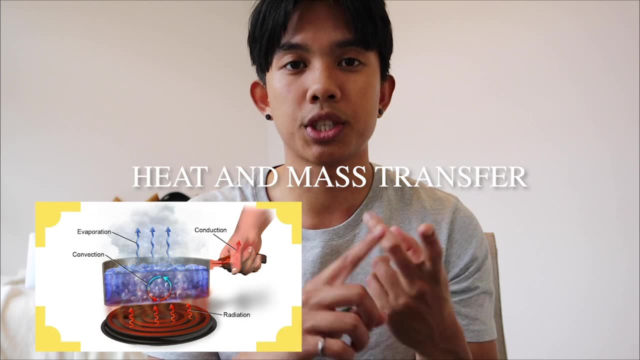 is certain operational techniques to make sure that they're always operating at their most efficient and safe region. Next up, we have heat and mass transfer. You'll learn about the different modes of heat transfer- conduction, convection and radiation- and then you'll apply those concepts. 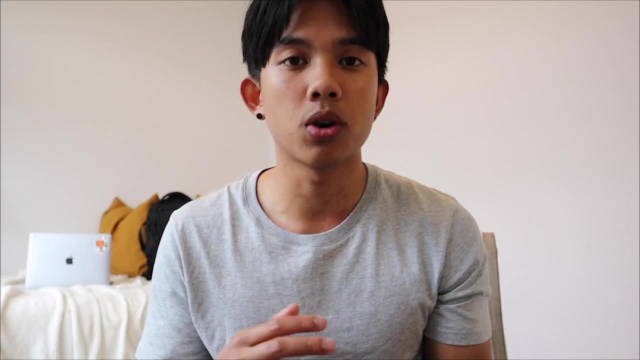 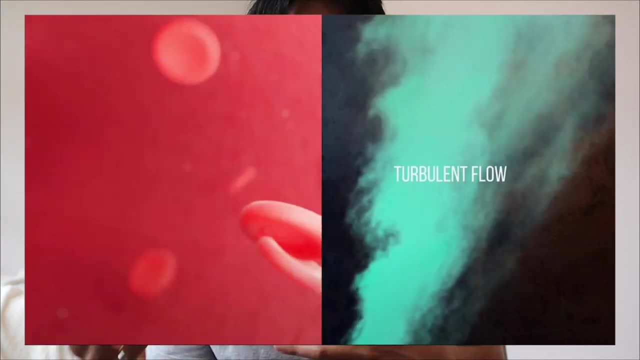 to design equipment such as heat exchangers. And lastly, one of our main courses is going to be fluid mechanics, which is learning about how liquids and gases move in systems. In this course, In this course, you'll learn about the different types of flow, such as laminar flow and turbulent flow. 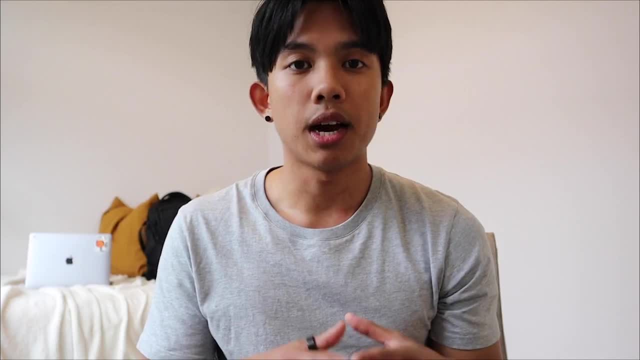 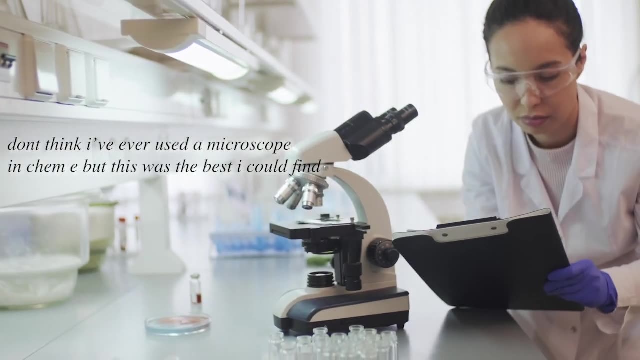 And you'll also learn about how to account for pressure drops in pipes. I think one of the most common misconceptions is that chemical engineering is all about chemistry. In my first year of general engineering, I took one chemistry course. In my second year, where I specialized into chemical engineering, I took three chemistry courses.